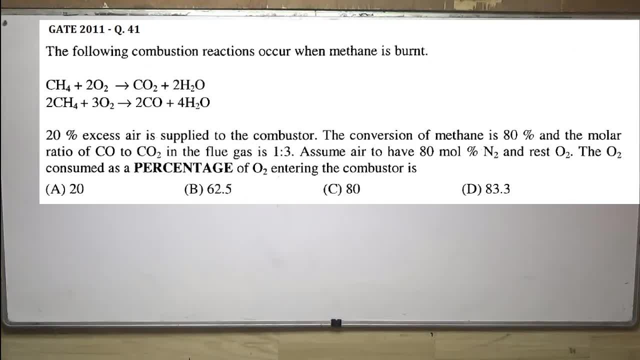 on the screen. It is given that the following combustion reactions occur when the methane is burned, That is, CH4 plus 2O2 gives CO2 plus 2H2O. 2H2O gives CO2 plus 2H2O- 2H2O. 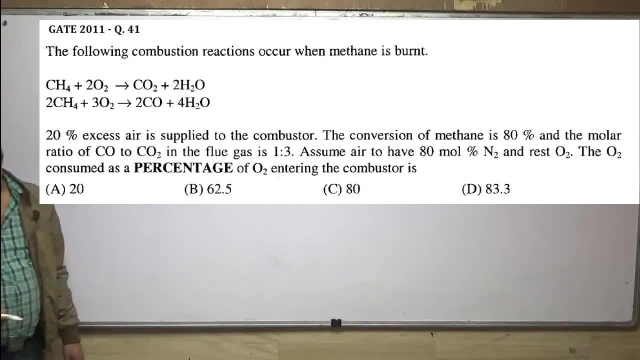 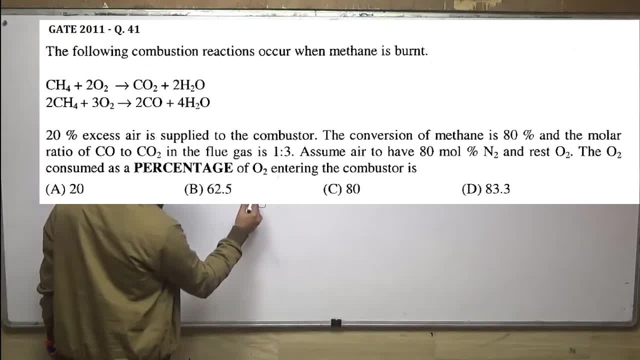 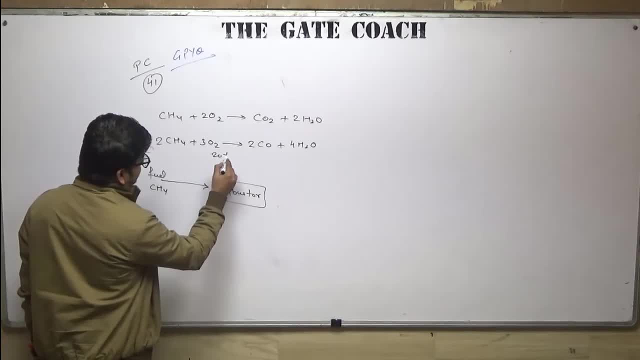 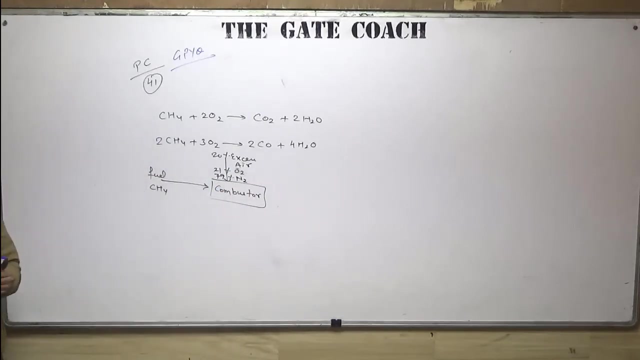 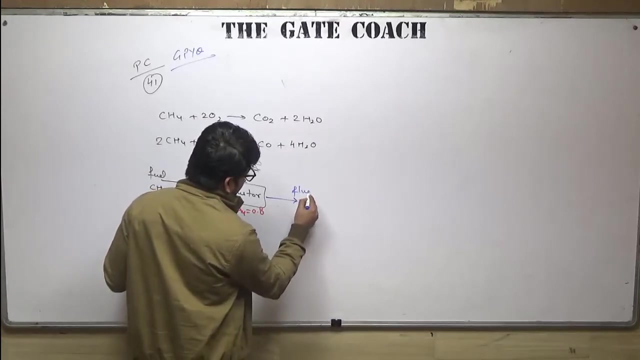 this is my combustor. This is fuel which is CH4 and 20% excess air we are supplying. We know that air has 21% oxygen and 79% nitrogen. The conversion of methane is 80%. The molar ratio of CO2CO2 in the flue gas is 1 by 3.. This is the flue gas: CO2CO2, its molar ratio. 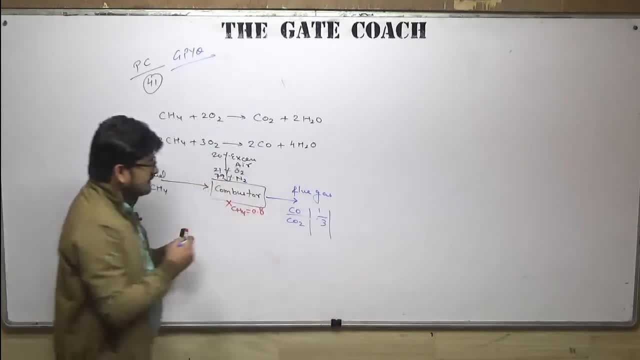 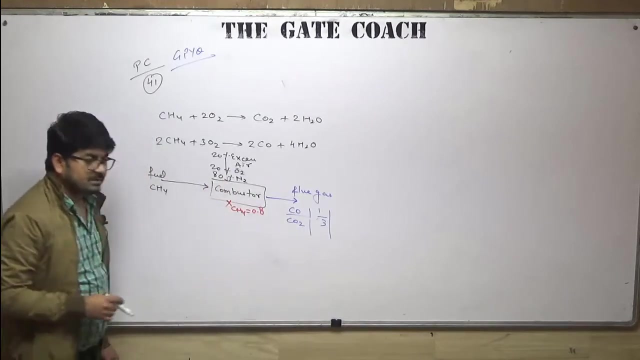 is 1 by 3.. In the product gas In this question we will take the given composition of air. It is not given by default. It is given that 80% nitrogen and 20% oxygen O2 is consumed as a percentage of O2 entered O2 consumed to the O2 fed percentage. This is asked by 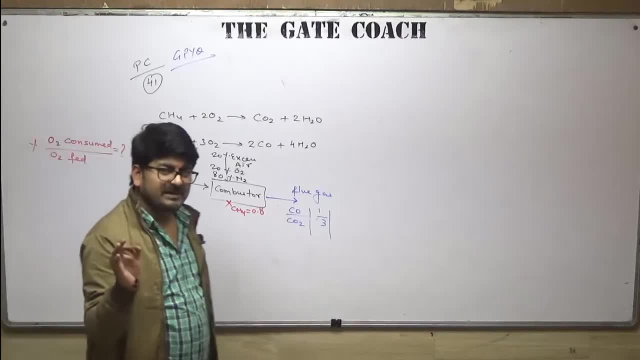 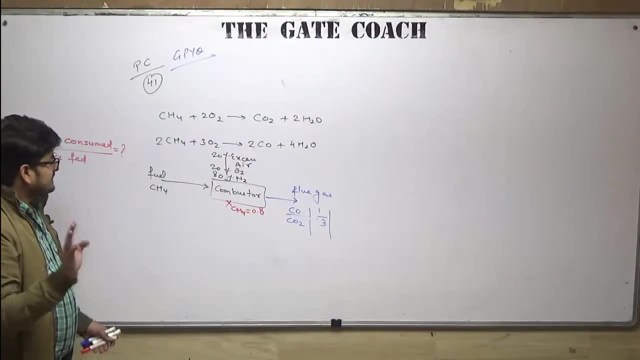 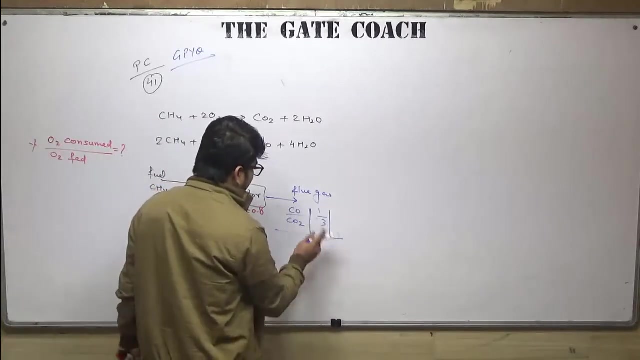 you material balance with chemical reaction flow, combustion fuel and combustion everything. just identify the components at the inlet. identify the components at the outlet. in the outlet I will have CO, CO2, H2O, oxygen, nitrogen and unreacted CH4.. 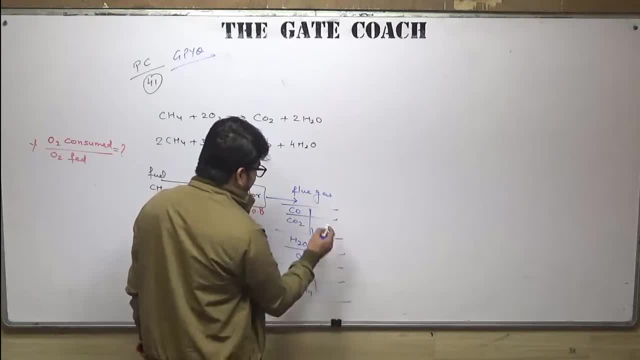 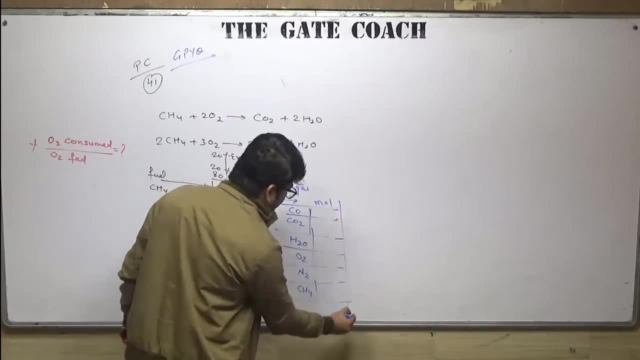 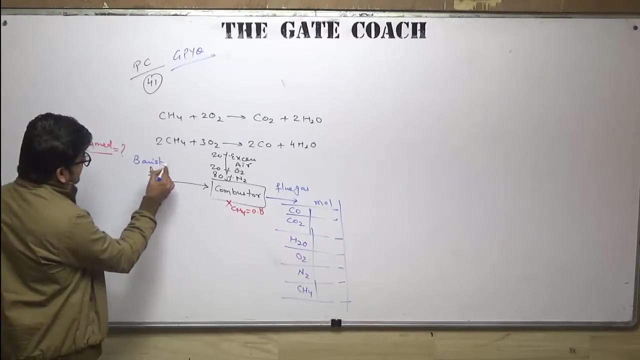 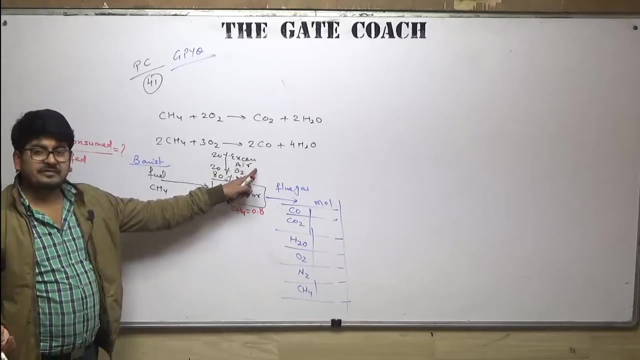 Suppose these are moles and we have to calculate their amount, identify the components and calculate their amount. Let's say my basis is because I have to find the percentage of O2 reactant. I have to tell, in respect to the input, how much air we have fed in excess. only then we can calculate. 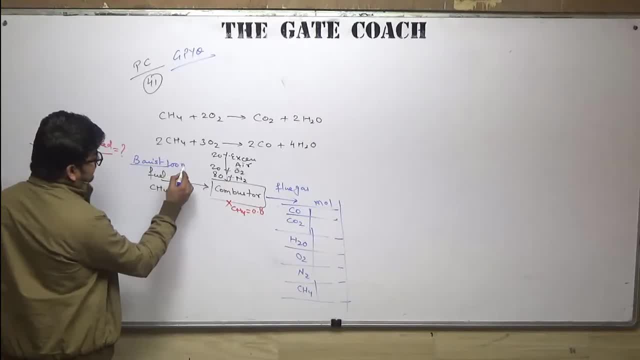 when we know the amount of CH4.. So let's say, my basis is I have to calculate the amount of CO2, CO2, H2O, oxygen, nitrogen, nitrogen and CO2, this is 100 moles of CH4 fed. 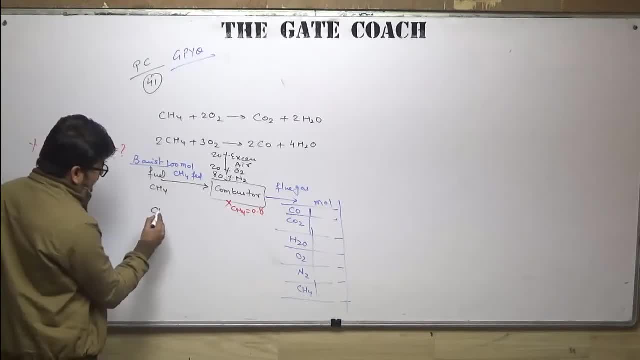 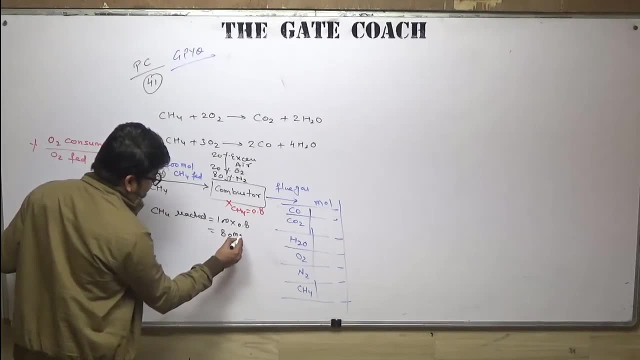 So here you are, given CH4 reacted 80%, so 80 moles. you have identified the components at the outlet and calculated the amount of CO2, so what is CH4? It is unreacted. Unreacted is 20 moles. 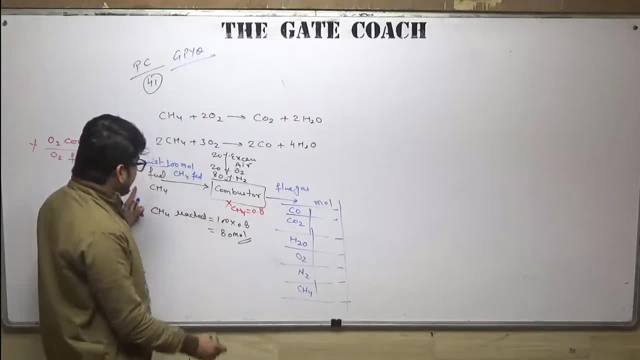 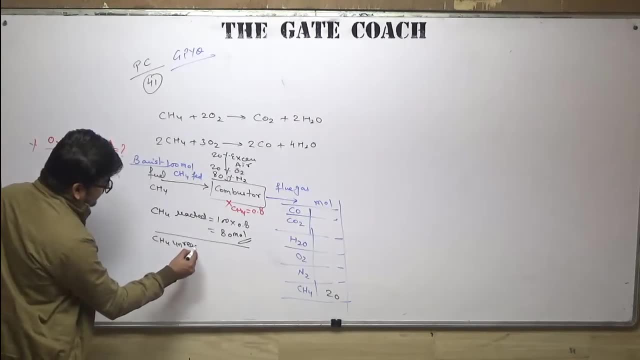 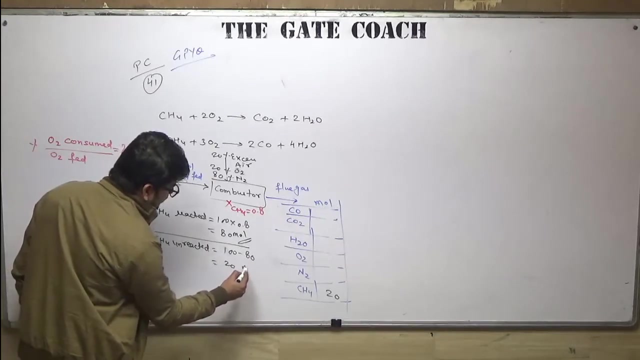 80 is reacting, so CH4 is unreacted. So what is CH4?? What is CH4? Reacted. So how much is CH4? Unreacted? unreacted will be 100 minus 80, that is 20 more now excess air. so calculate the amount. 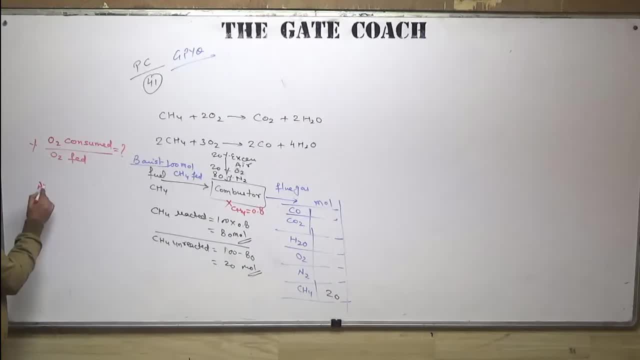 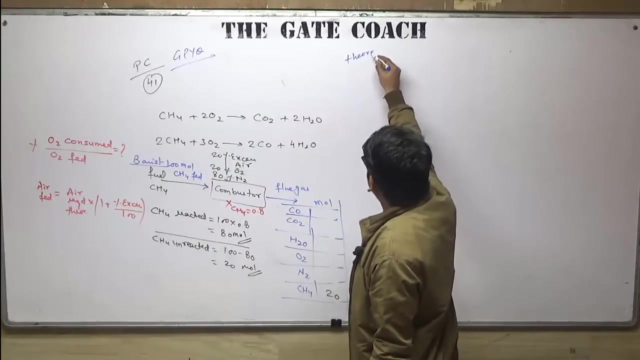 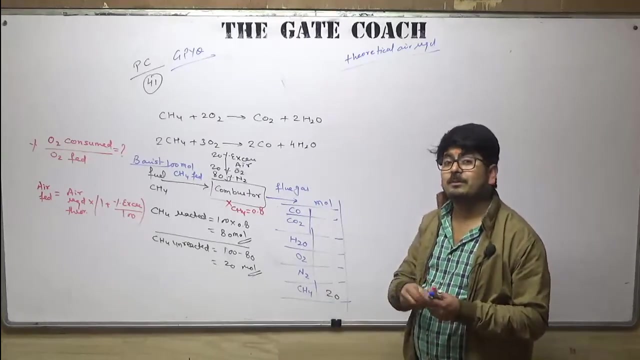 of air that I have fed. so I know that air fed is air required theoretically multiply by 1 plus percentage excess over 100, so I will get my answer. so theoretical air required we calculate for complete conversion and complete combustion. operating conditions doesn't matter. 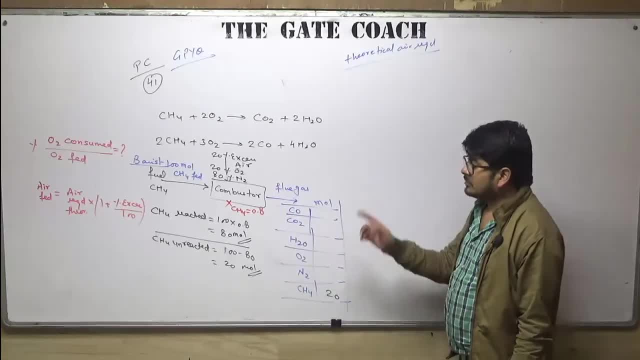 complete conversion and complete combustion. we calculate. So see, I have calculated the amount of air that I have fed. so I know that air fed is 100 plus percentage excess over 100, so I know that air fed is 100 plus percentage excess and complete combustion of 100. 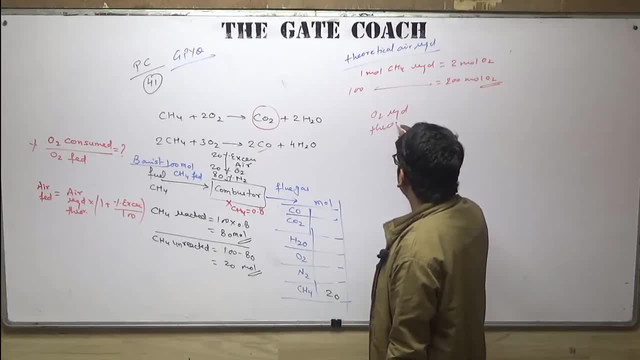 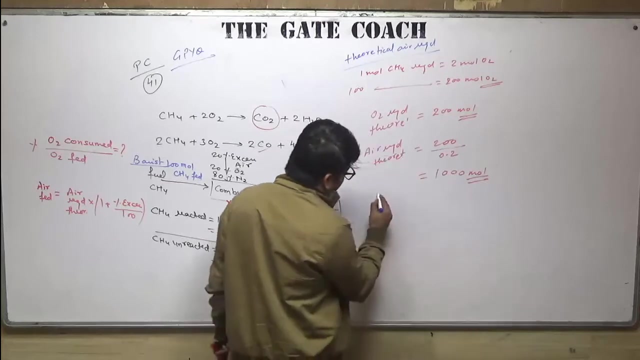 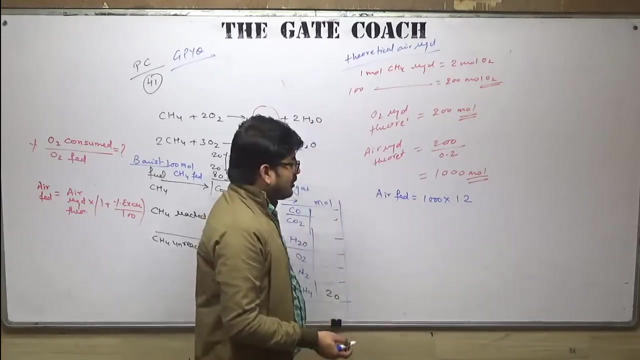 So no, consider yet. so complete combustion of 100 would be 100 plus percentage excess, 200 moles. So air required theoretically will be 200 over 0.2, that is 1000 moles. It means air fed air required theoretically multiplied by 20% excess, so 1.2, 1200 moles. 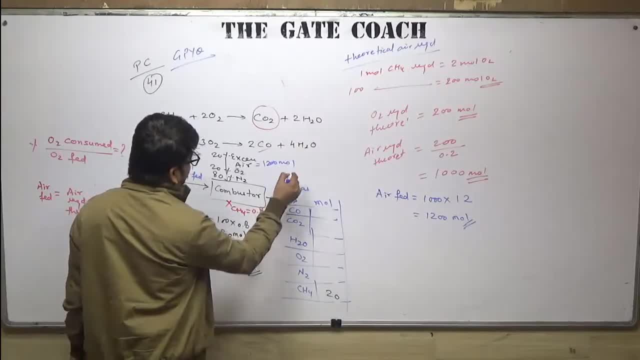 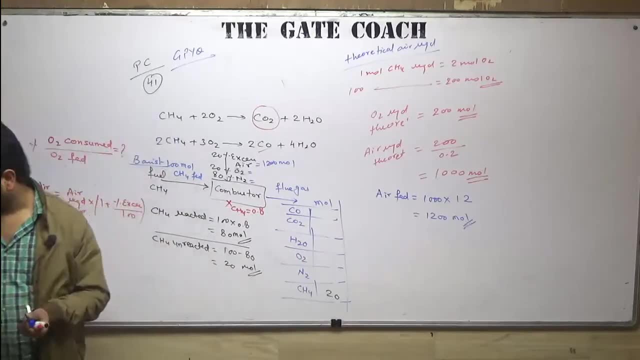 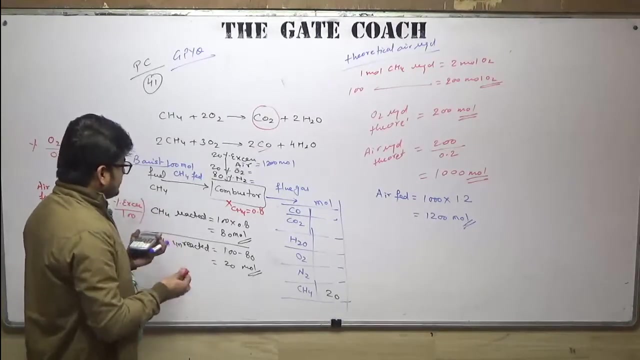 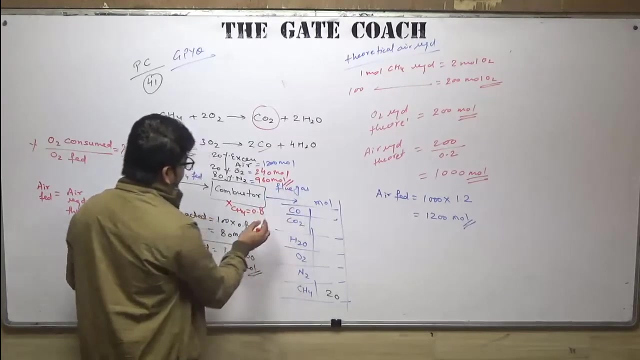 So air fed is 1200 moles, in which how much oxygen will be there, That is, 1200 into 0.2 moles. Oxygen fed will be 240 moles and nitrogen fed will be 960 moles And the amount of nitrogen 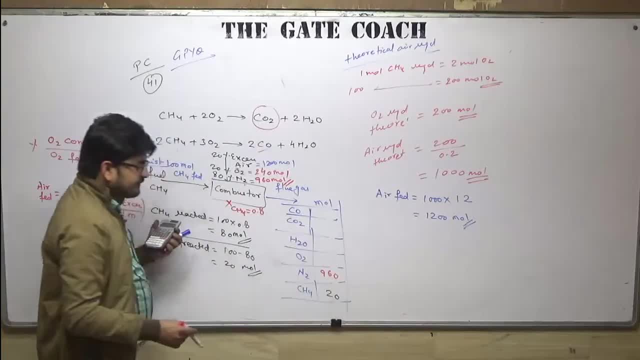 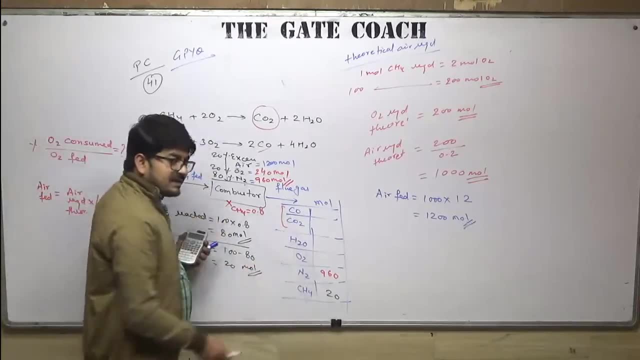 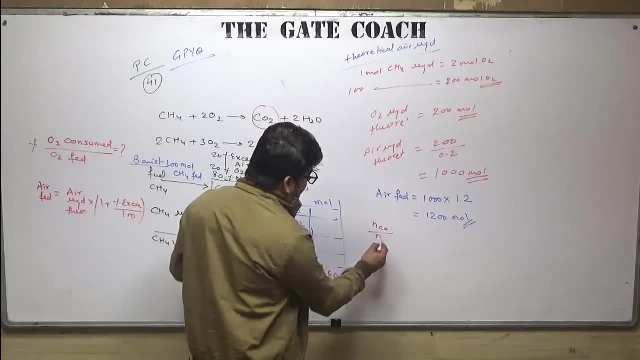 और आत्यानल में आपको दिग्या है कि moles of CO divided by moles of CO2 in outlet is 1 by 3.. 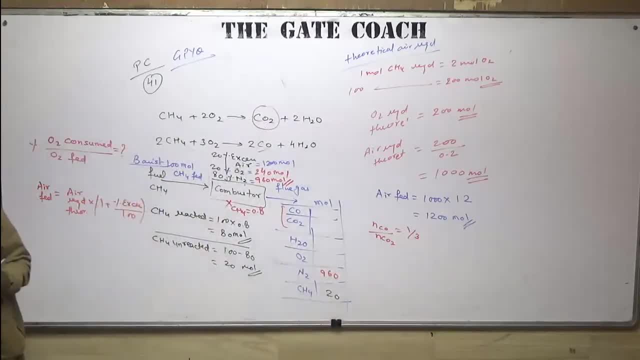 महानम जदाना भी CO2 बन रहा है. एक बाँ में फिर से निभर करेगा. 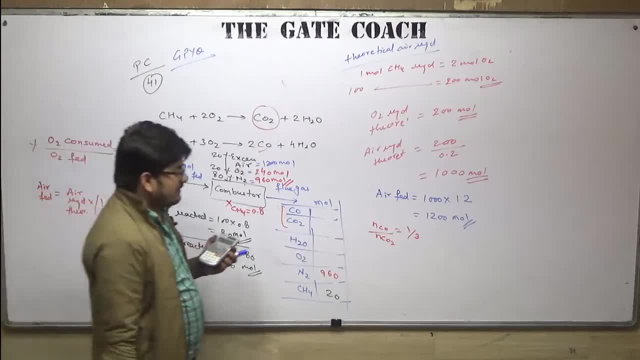 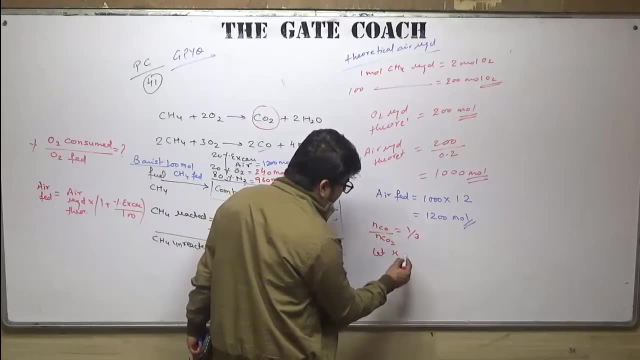 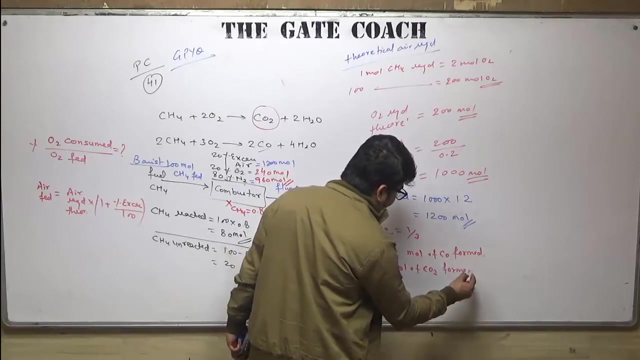 लेता हूँ moles of CO2, moles of CO2 in flue gases, 1 by 3.. So it means, suppose I take let x moles of CO formed, so moles of CO2 formed will be. 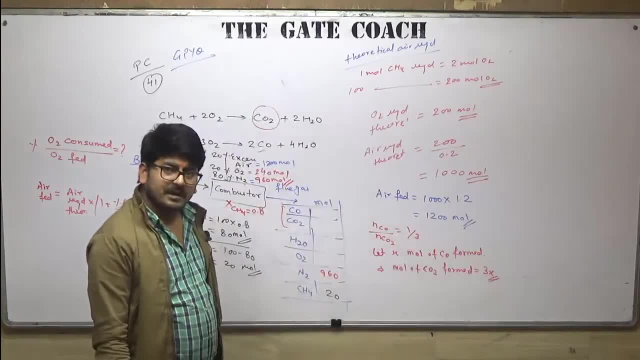 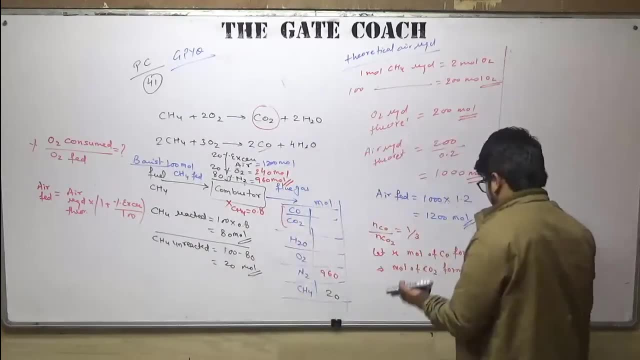 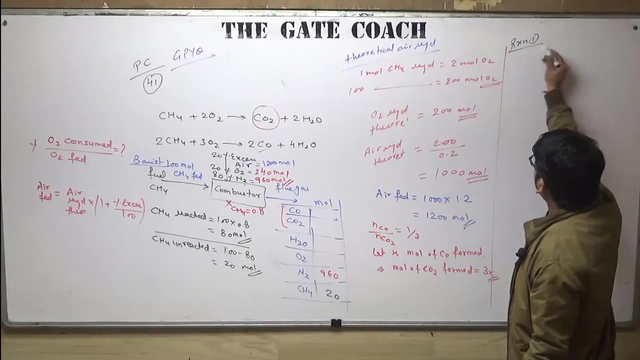 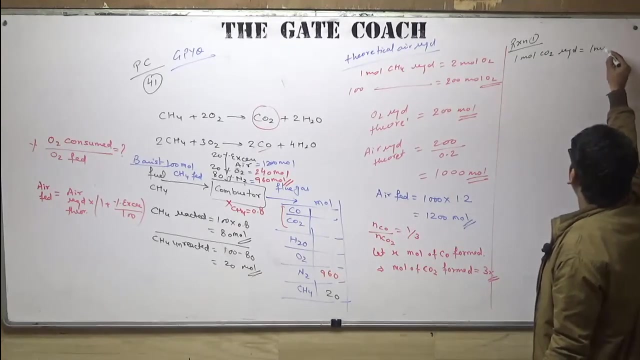 3x. If x moles of CO is formed, then how many moles of CO2 will be formed? 3x. Now you see, from reaction 1, it is clear that 1 mole CO2 required 1 mole of CH4.. So 1 mole of CO2. 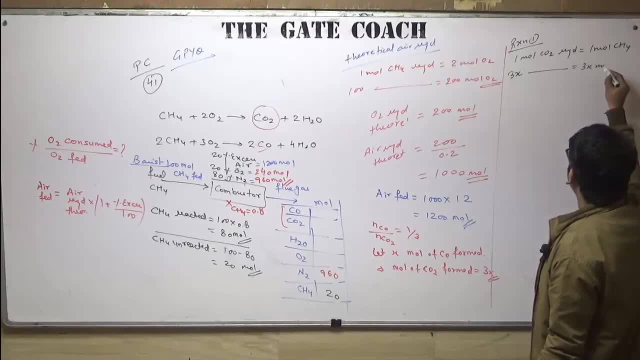 required 1 mole of CH4.. So 1 mole of CO2 required 1 mole of CH4.. So 1 mole of CO2 required 1 mole of CH4.. So 3x moles of CO2 will required 3x moles of CH4. Simple, And 1 mole CO2 required 2 moles of oxygen. 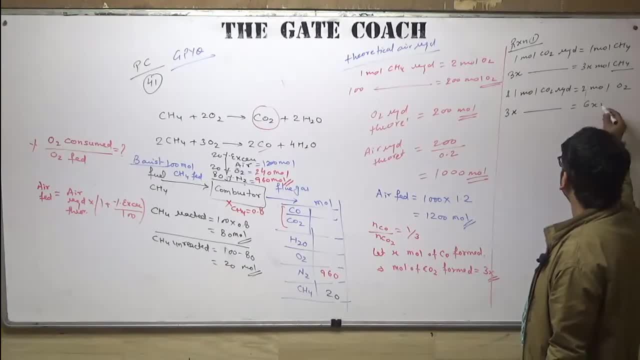 So 3x moles of CO2 will required 6x moles of oxygen. Ok, Now let us come to reaction 2.. In reaction 2, it is clear that 2 moles of CO required 2 white moles of CH4.. 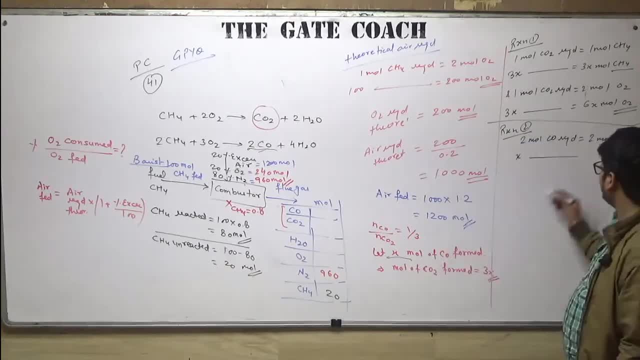 So x mole of CO- we had assumed in X mole in the outlet will require X moles of CH4. Number 2. C questions are given as lizuzan Tran Shot. then I guessed that 2 moles of CO resources. 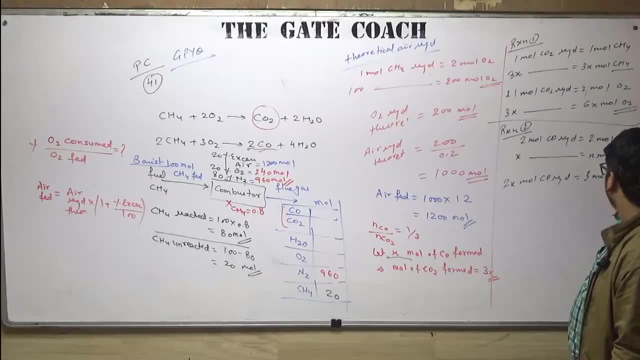 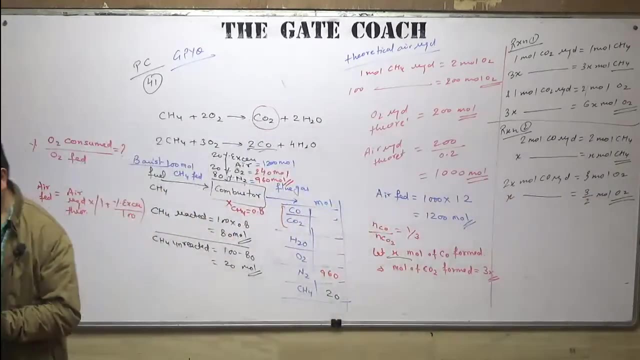 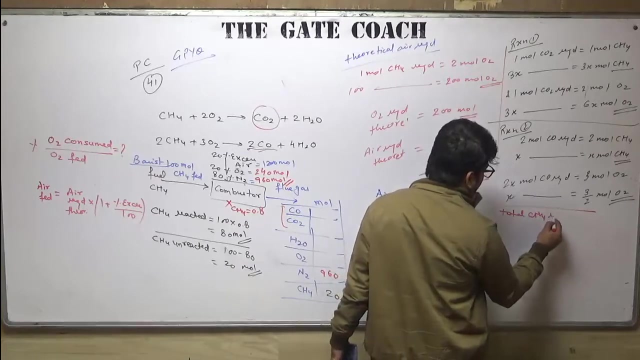 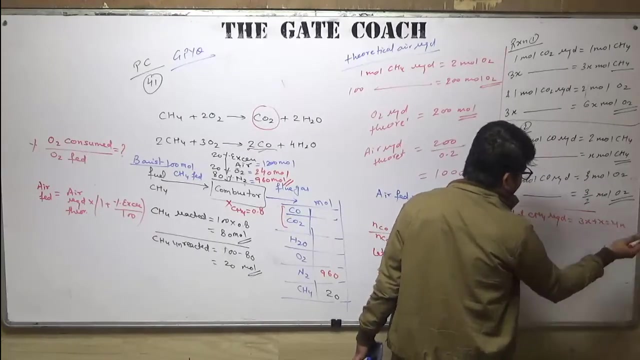 required 3 moles of CH4, sorry, oxygen. so x moles of CO will require 3 by 2 moles of oxygen, simple. So here you can see that total CH4 required will be 3x plus x, equal to 4x. that means: 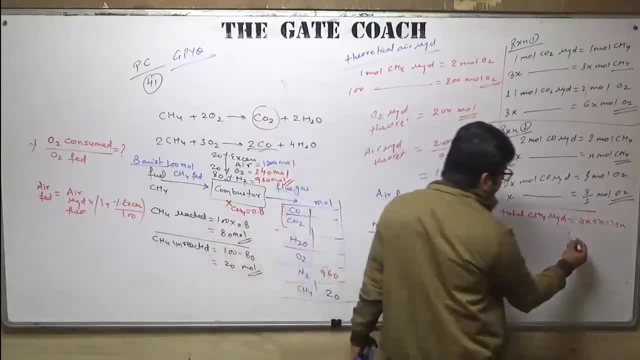 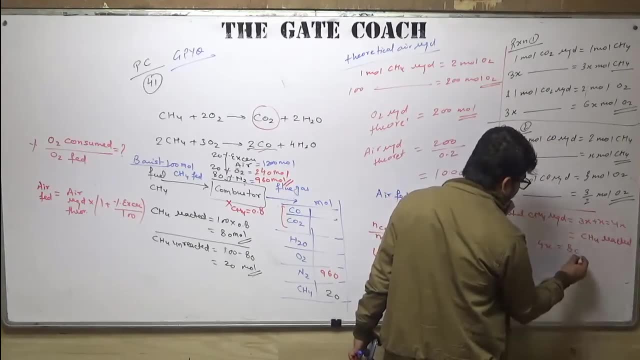 this much CH4 is required for this reaction and this value of reactance should be equal to CH4. reacted means 4 x equal to 80, because 80 moles of C should be equal to 30 moles of reactance. 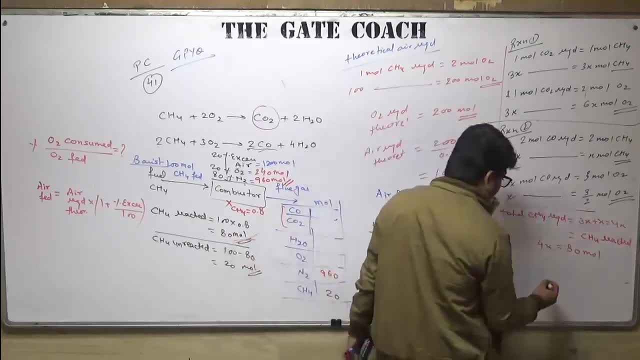 So we are going to be writing the value of reactance. So we are going to write the value of reactance. So we are going to write the value of reactance. CH4 is reacting. We have seen this. So X equal to will be 20 moles. This means how much? 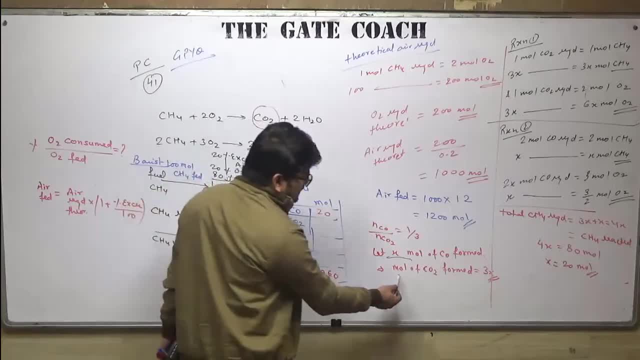 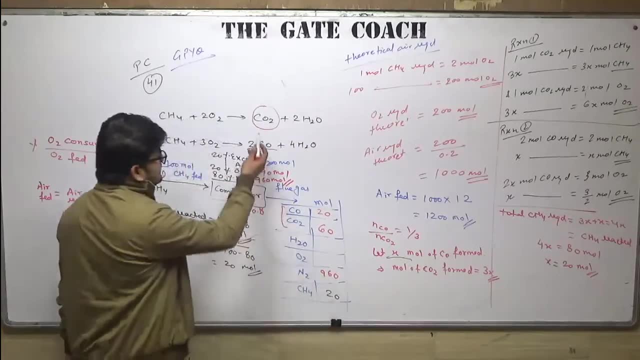 CO is there in the outlet? 20 moles. How much CO2 is there? 3X, That is 60 moles. Now S2O and oxygen S2O need. You can calculate S2O in the same way, But here there is no need. 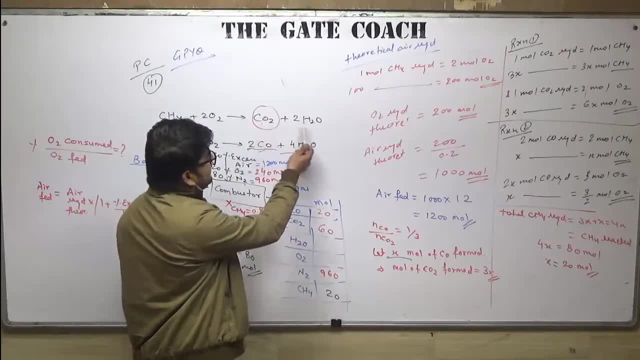 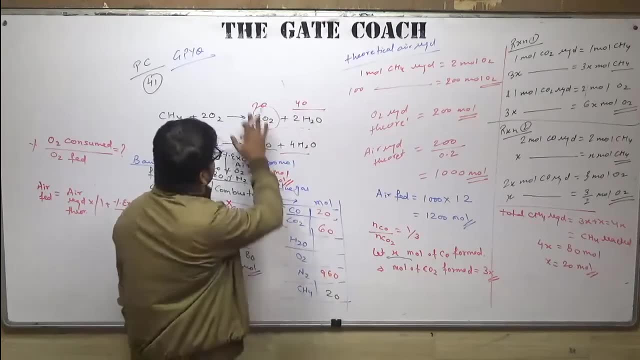 so we are not doing it. Otherwise, you know, 1 mole CO2 formed with 2 moles of S2O. So 20 moles of CO will formed along with 40 moles of S2O. Sorry, 60 moles of CO2 formed. 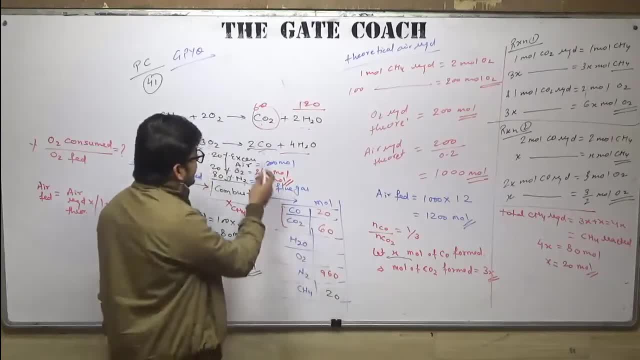 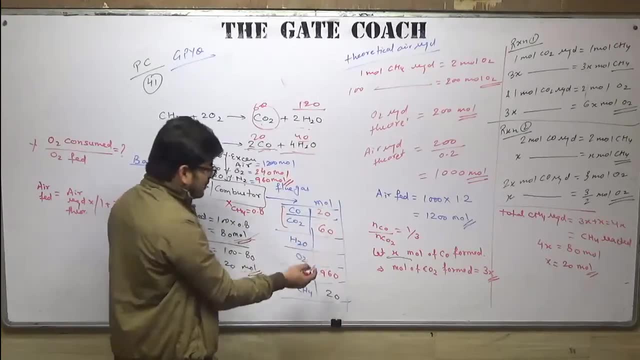 along with 120 moles of S2O. Okay, 2 moles CO formed with 4 moles of S2O, So 20 moles of CO will formed with 40 moles of S2O, So total S2O formed will be 160.. How much oxygen? 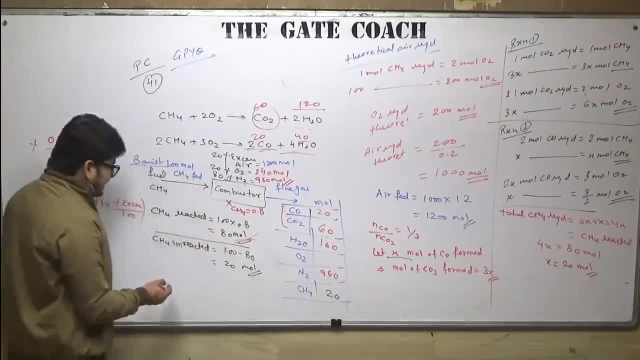 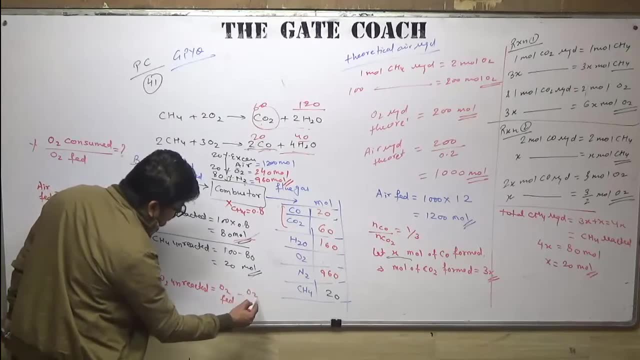 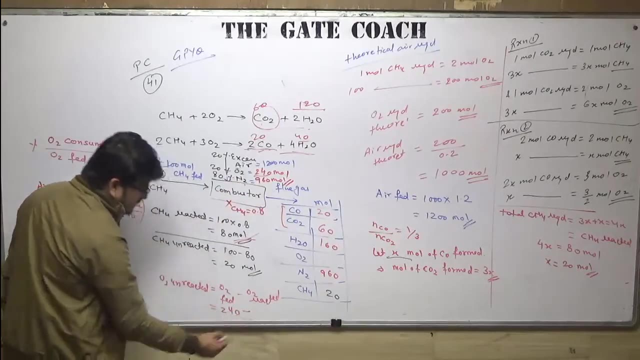 will be there. This oxygen will be unreacted. Unreacted means O2 will be unreacted. O2 will be fed, minus O2 is reacted. How much O2 is fed? 240 moles O2 is reacted. How much oxygen? 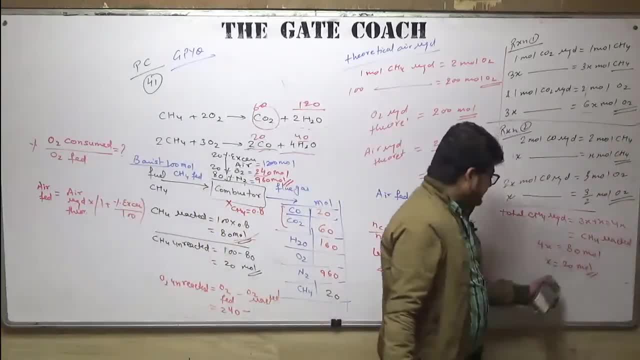 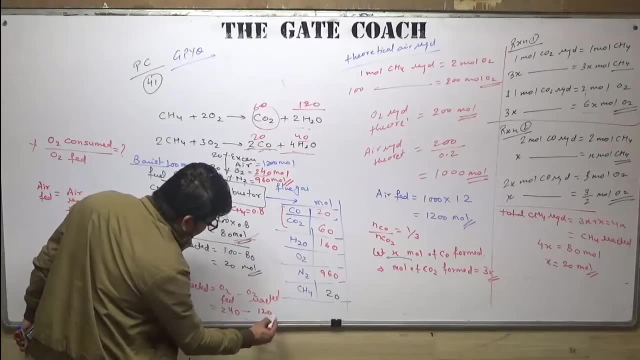 is being reacted. in the first reaction, 6X, The value of X is 20.. In the first reaction, 6X, small oxygen is being reacted, So this value will be 6 into 20, 120 minus O2 is. 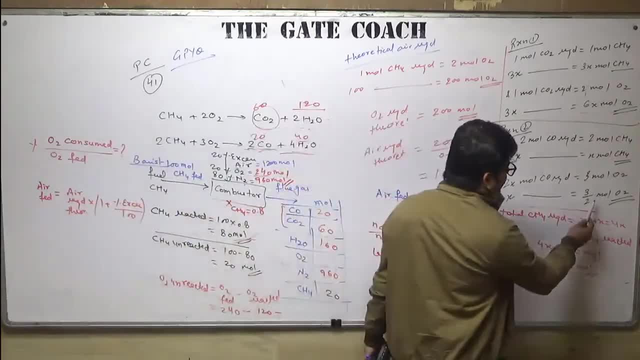 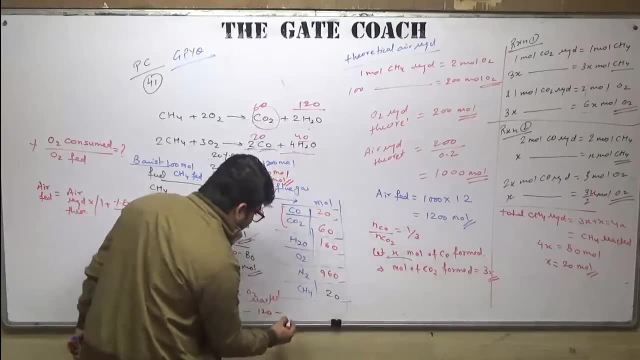 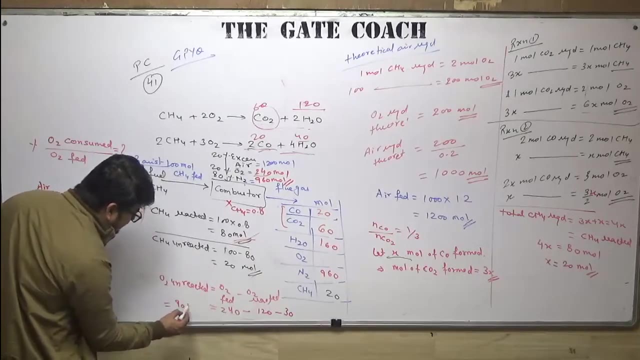 being reacted in the second reaction. In the second reaction it is 1.5X. The value of X is 20. So in the second reaction oxygen will be 30. So my oxygen will be unreacted 240 minus 150, that is 90 moles. Okay So. 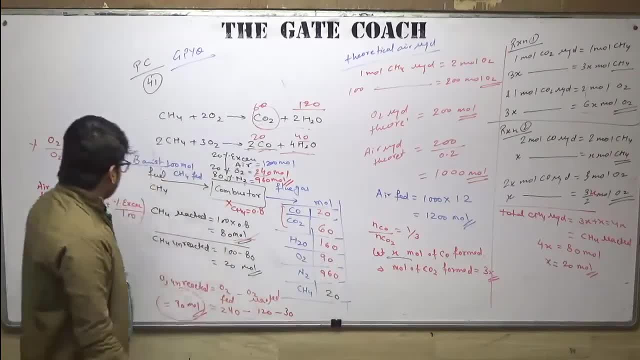 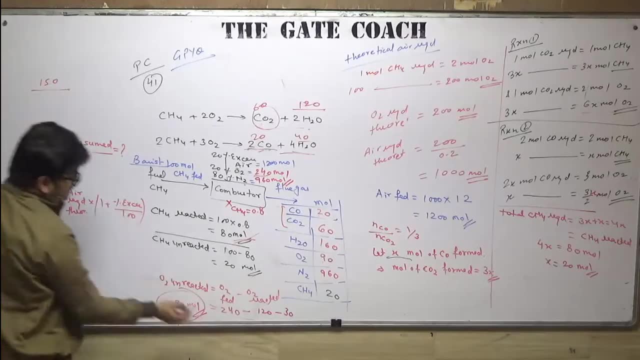 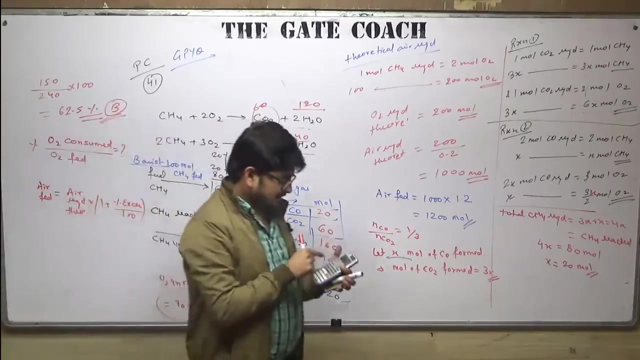 here I have 90 moles of oxygen. So what will be the answer? How much O2 is consumed? 150, 120, 120.. 20 plus 30 divide FAD into 100, that is sorry, that is 62.5%. So option B will be your answer. 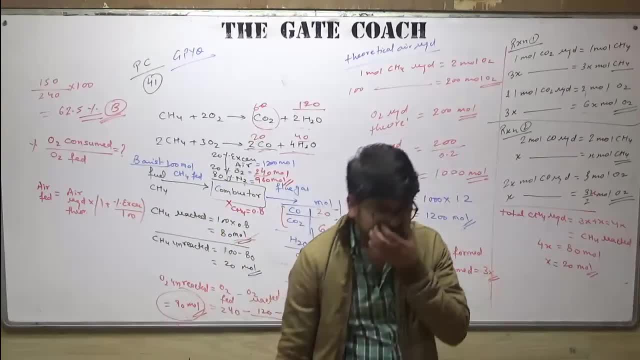 Simple, So simple. See, to solve the problem of material and energy balance, you don't have to do anything big. You just have to keep in mind one thing: You just have to be careful. You just have to be careful. You just have to start from the beginning. So this is the 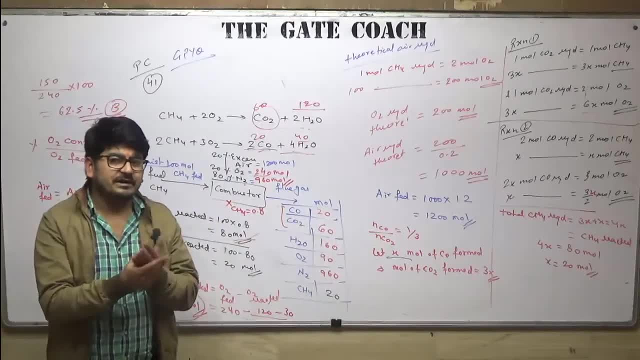 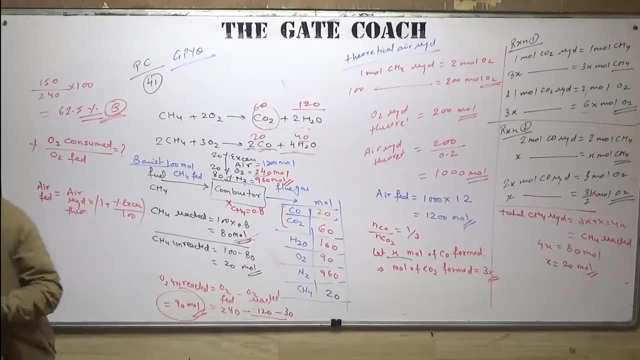 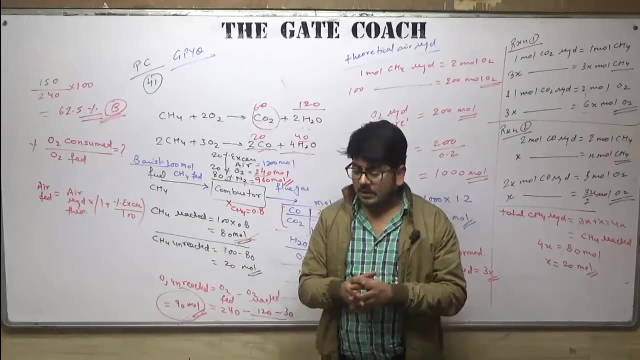 that you should have a single approach to solve the problem. if you see the books, there are n number of books available in the market. there are n number of books available in the market. and if you see in the books, different approaches are given to solve different questions.